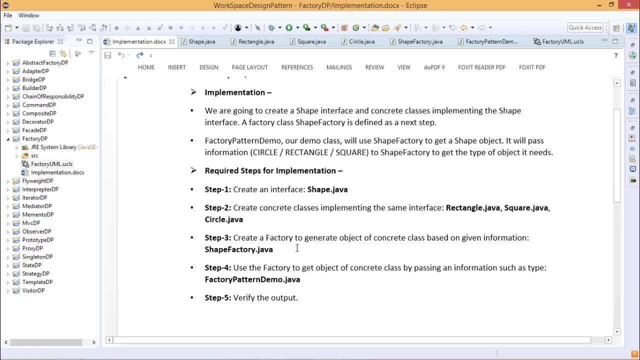 interface And then we will be going for create a factory to generate the object of concrete class based on the given information. So, depending upon the input argument, the respective object will be created And use the factory to get the object of concrete class by passing. 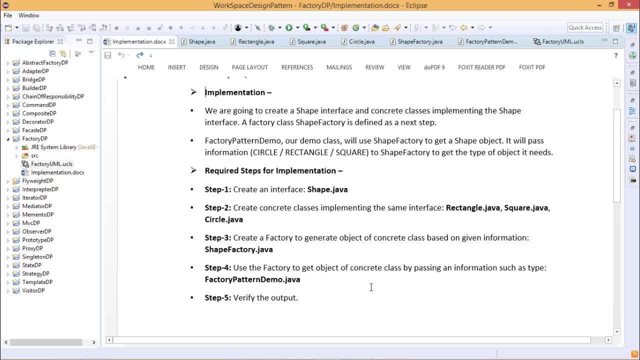 an information such as the factory pattern, demojava, And we will be going for the verification of the output. So let us go through the steps at first. So here we are going for the steps. So at first we are having this shapejava, So public. 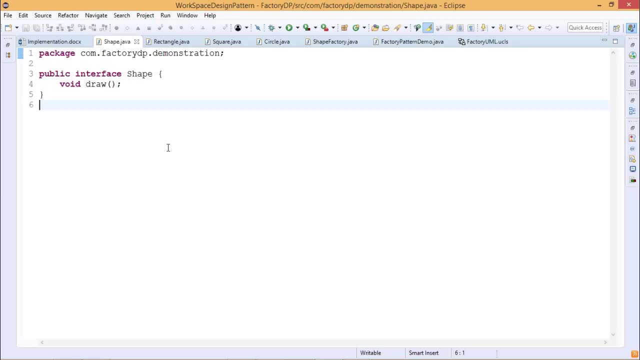 interface shape and it is having only one method. that is the draw. Next, we are going for this concrete class, So that is the public class rectangle implements shape. So this particular shape is nothing but the interface which has got implemented by the class rectangle. 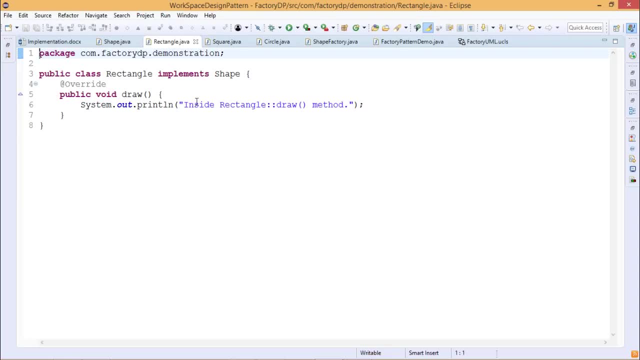 So this draw method is having its body. So that is the inside rectangle, colon class. Similarly for the square also, it is implementing the shape interface and draw method has been defined as it is on the screen. We are having the circle also. We have done the same thing. 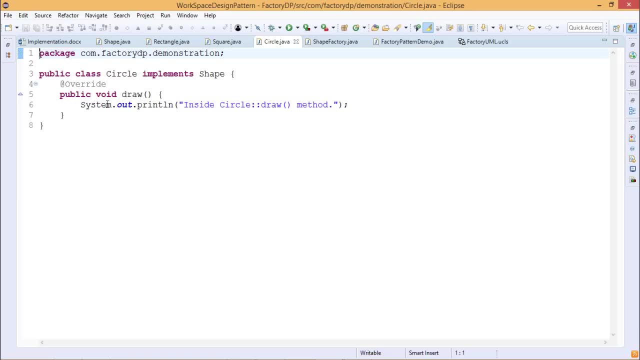 that is, circle is implementing the shape interface and the draw method has got its body. So now we are having this shape factoryjava. In case of shape factoryjava, we are having one method, The name of the method is get shape, And it is taking one string as input. 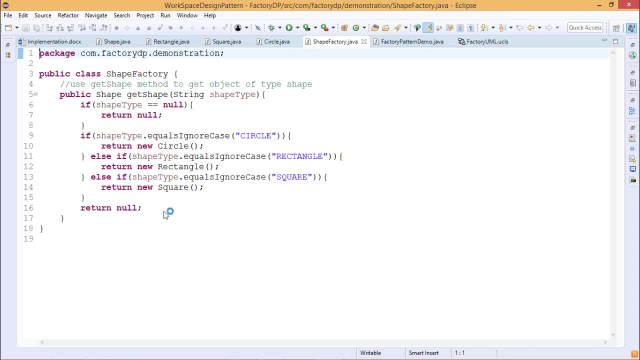 argument And it is returning the shape object as output. So, as that is why you have written this, one is return argument is shape object. So when this input string that is a shape type is null, it will return null. But when the shape type dot equals, ignore case circle. So it 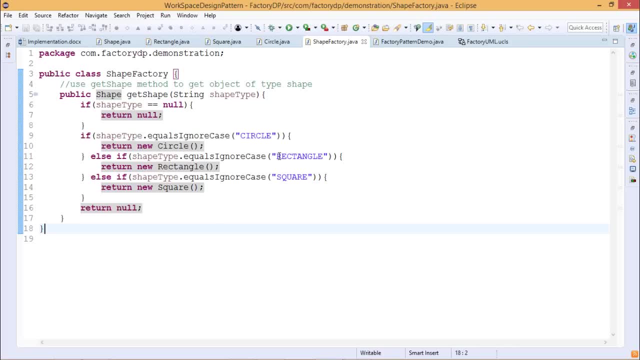 will be returning the circle class object. In case of rectangle, if the input string is rectangle, then it will return the rectangle class object. So, new rectangle constructor And whenever we are passing this square as a input, We are having a new rectangle constructor. 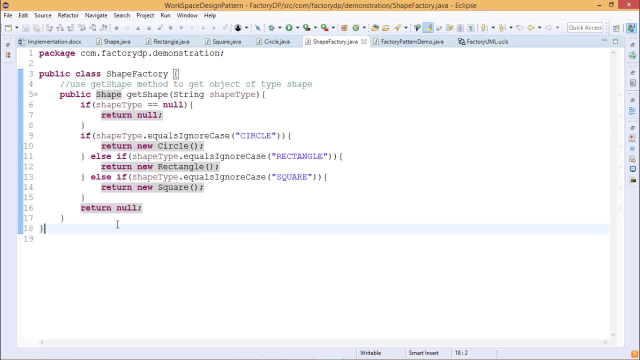 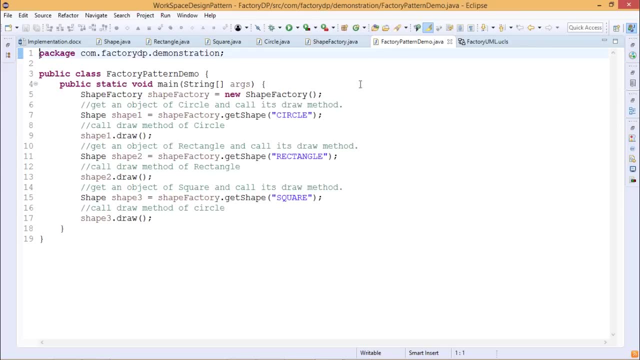 input argument. so it is returning the square class object as output. otherwise it returns null. otherwise, okay, now we are going for this factory pattern demo dot java. so in this factory pattern demo dot java, we are defining shape factory object, that is, the shape factory is equal to new shape. 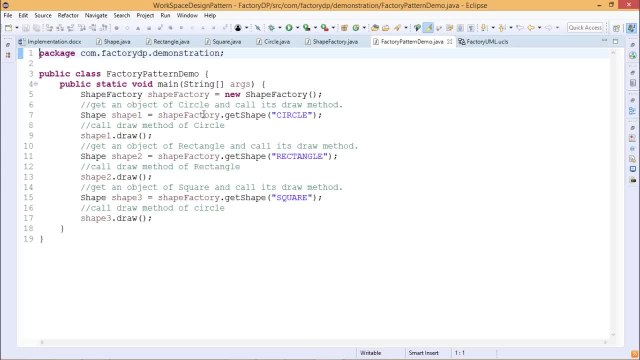 factory constructor. so shape shape one is equal to shape factory dot. get shape circle. so you see, here we are passing one, the circle as the string, as input argument, and that's why it will create the circle class object as output, and that is initializing this shape one. so when you are 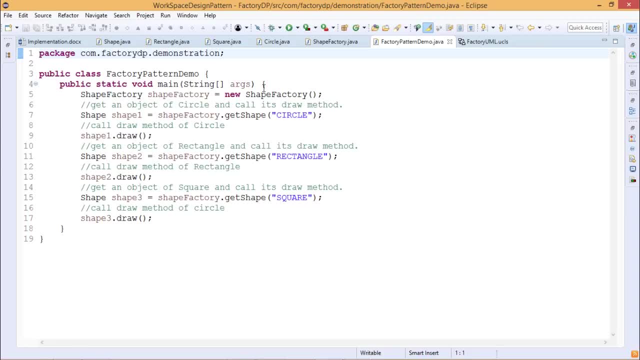 writing this shape, one dot draw method is getting initiated- will be getting the required output. so now i'm just showing you the output here. so now it is printing the inside circle colon colon draw method, so that very method which was defined under the circle class is getting executed. but 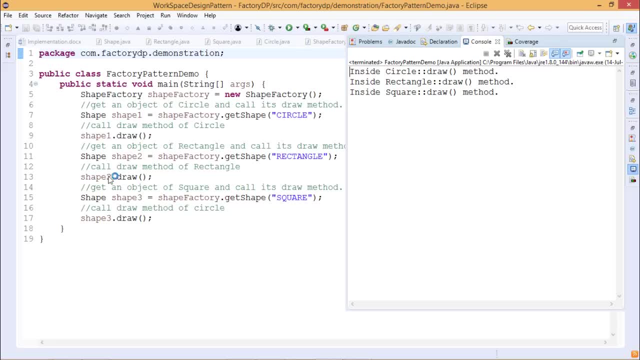 when you are passing this rectangle and we are writing this, we are calling this method draw. that is a shape, two dot draw. it is calling the draw method which was defined under the rectangle implementing class. and when you are passing this square as input argument, then it is returning, it is just executing. 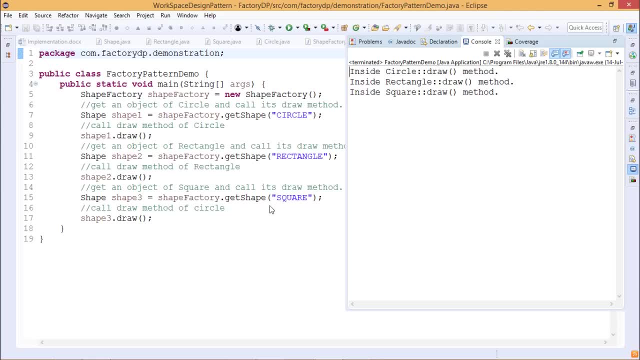 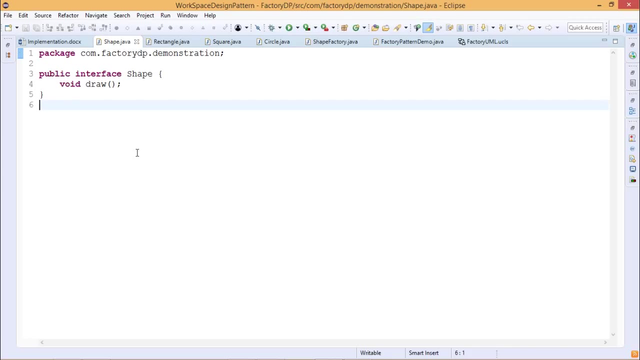 uh, that draw method which was defined under the square, under this particular square dot java, which is implementing the shape interface. so in this way we are getting this record output. so let me revise once again. so this is my shape dot java. that is one interface having one method without body. 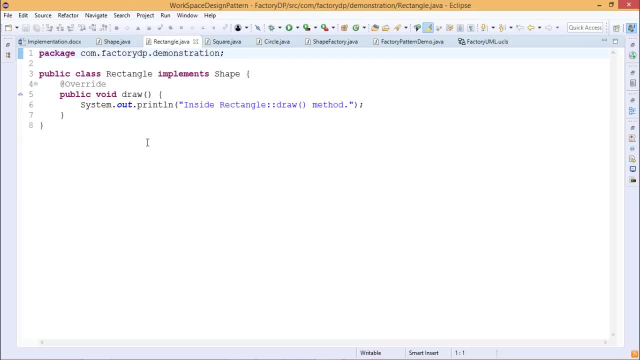 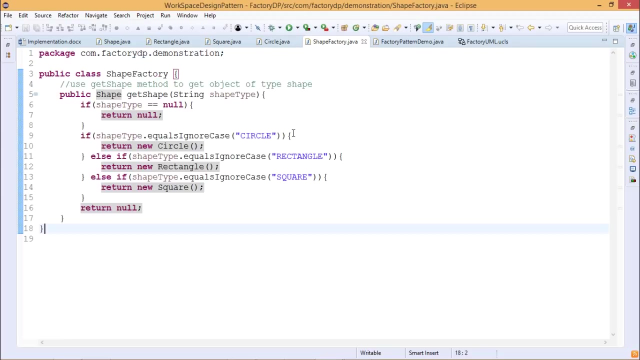 that is the draw method. rectangle is one of the implemented classes implementing classes of the shape interface and square is another class implementing shape interface. circle is another class implementing shape interface and respective draw method is having the body accordingly. shape factory is this one, so it is just returning the shape object, self interface object as output. 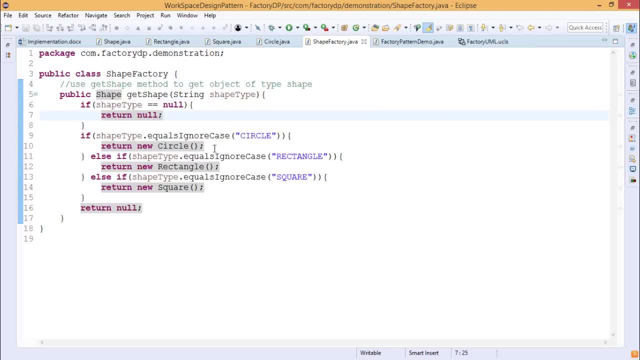 it takes a string as input argument. depending upon the string, whatever we are passing, the object will be returned. so when, when we are passing this circle as input argument string, it is returning the circle class object as the return type. so in case of rectangle, new rectangle constructor. in case of square, we are having return new square constructor. otherwise it will return. 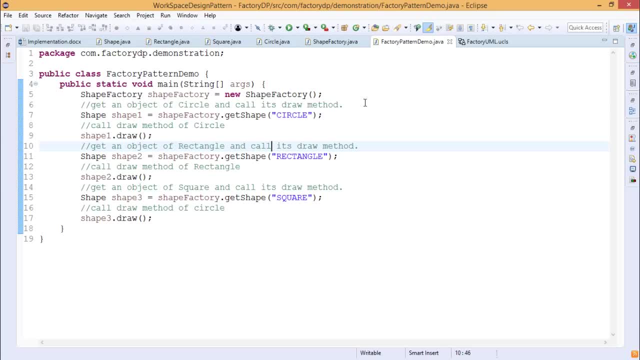 null. so in case of factory pattern demojava, whenever we are calling we are defining one shape, one on object under the shape interface and is equal to shape factory dot get shape circle. so now, when you are passing this circle, then circle class object will instantiate this shape.